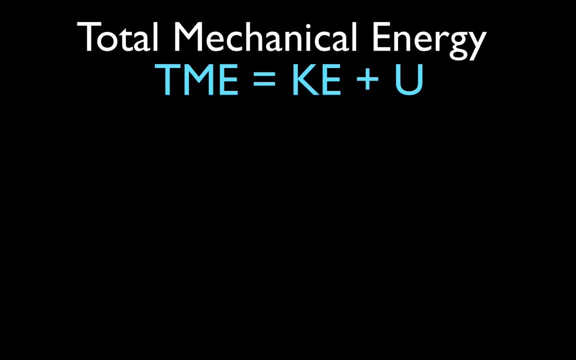 Now we want to use this idea of total mechanical energy and put it together with conservation of energy. so we can have conservation of mechanical energy, Because we like to say that if we have a conservative system, a system where only conservative forces operate, a system where the energy is being conserved, we have a special system, a conservative system. 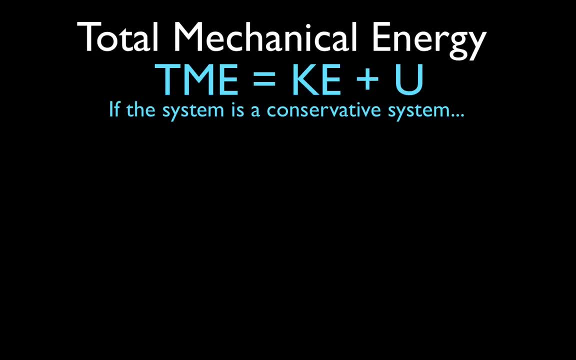 Now, what kind of system is a conservative system? Basically, I like to think of it as a system where there is no friction. That's a good rule of thumb. Friction is a non-conservative force. It's taking energy out. 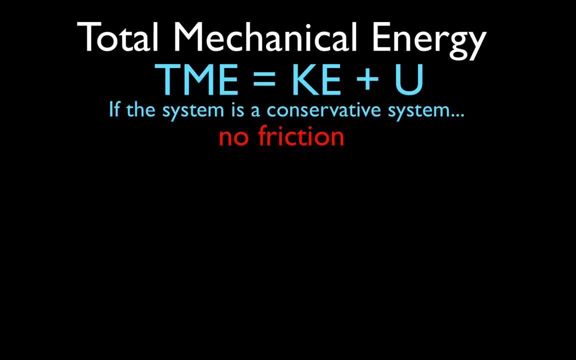 If you think of Newton's first law of motion: objects in motion stay in motion. Well, we don't really see that that much on Earth, because we're all We're always fighting friction. Friction is the thing that takes energy out, that slows things down. 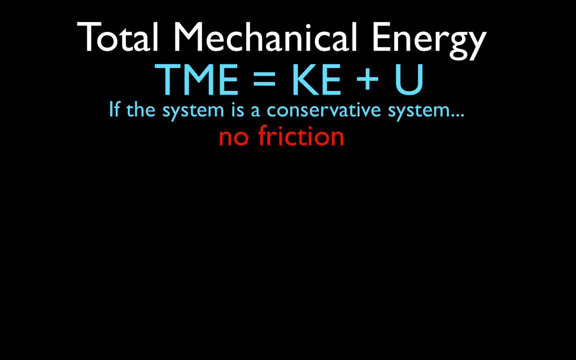 So in a conservative system there's no friction. But if we say the system is a conservative system, then the sum of the kinetic and the potential energies, the total mechanical energy, is a constant and equals the total mechanical energy of the system at any time. 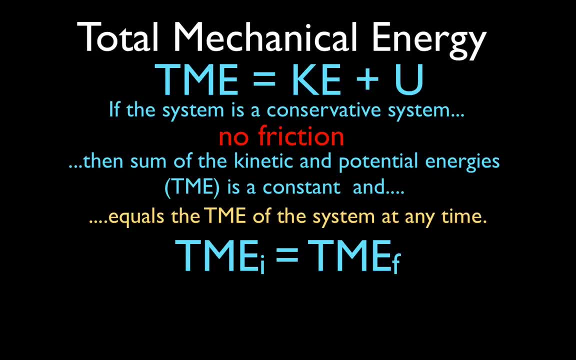 So then we can say that the initial energy equals the final energy- Conservation of energy- And we can expand that, and this is the equation we like to use. We like to say that the initial kinetic energy plus the initial potential energy is equal to the final kinetic energy plus the final potential energy. 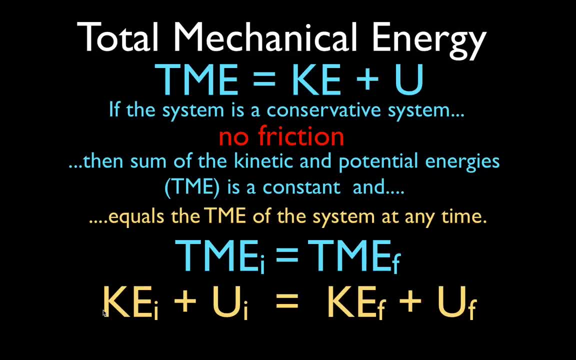 That statement is true. if we have conservation of energy within our system, That means we have to have a conservative system and we have to have no friction. Okay, Because friction is going to be taking energy out of the system. So this relationship is very important. 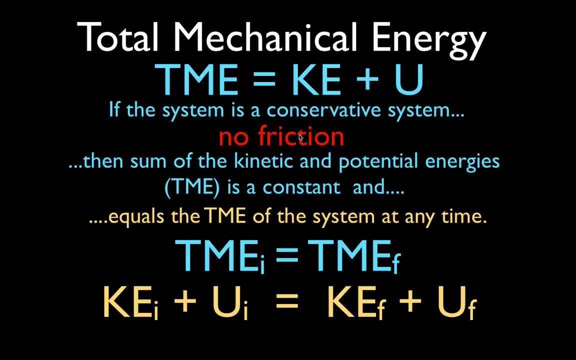 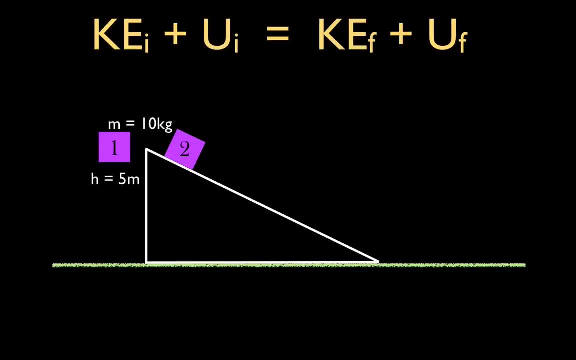 It's valid for a system that is a conservative system and has therefore no friction. Okay, Now let's go on and show you an example of how we use this idea of conservation of mechanical energy. We have two objects: object 1 and object 2.. 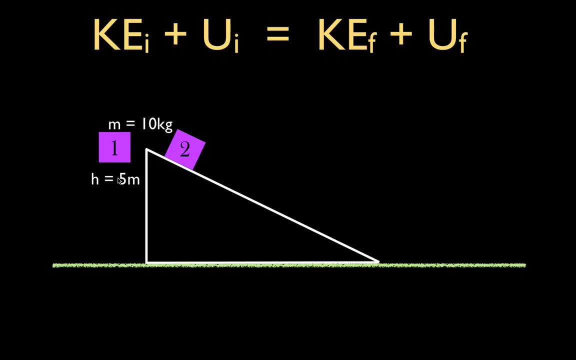 They're both standing still, They both have a mass of 10 kilograms and they're both 5 meters off the ground. Okay, And we are going to say that we have a conservative system, What does that mean? There is no friction. 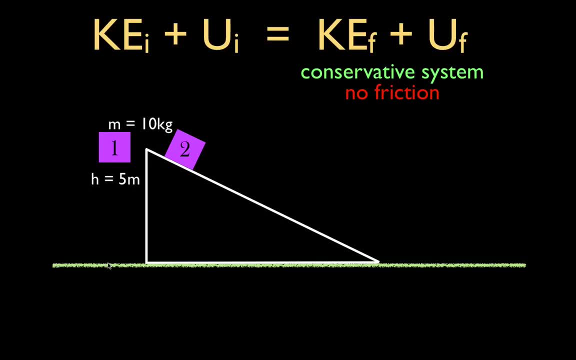 No friction Because we're going to allow this object to fall down towards the surface, No air resistance. We're going to allow this object to slide down this incline plane And we're going to say there's no friction between the object and the plane. 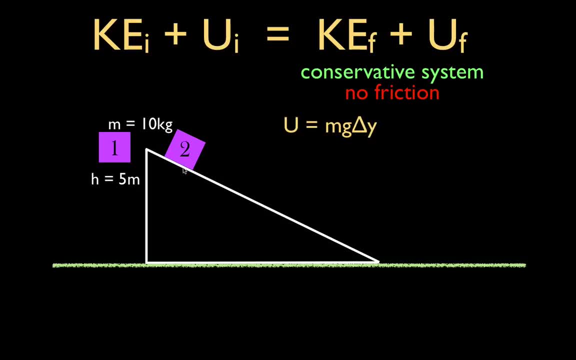 All right, Now let's remind ourselves our equation for potential energy and our equation for kinetic energy, And we want to keep those two things in mind. Okay, Now we want to, for this problem, determine the initial kinetic energy, The initial potential. 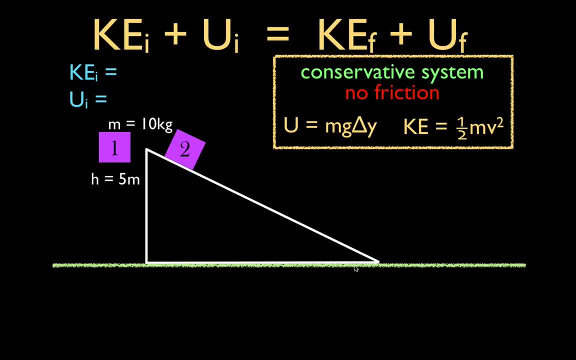 And then, after both of these things fall down or slide down, we want to find the kinetic energy final and the potential energy final And we want to see how we're going to solve those or answer those four questions and see if we can use conservation of energy to do that. 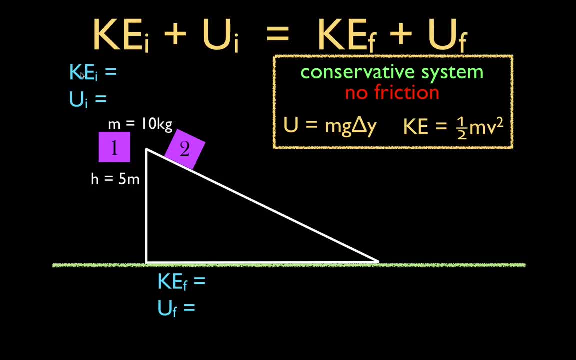 Okay Now, first of all, both objects are not moving. Okay, Both objects are not moving. That means that their velocity is zero. So kinetic energy is one-half mv squared. Well, if v is zero, then it should be pretty straightforward that the kinetic energy of both of those objects is zero. 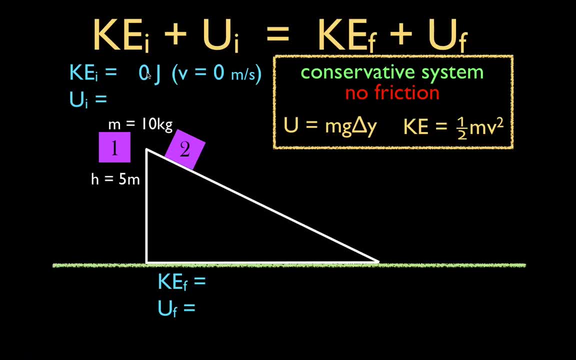 Okay, So we write down kinetic energy: zero joules. Now they do have some height above the surface And we can use this equation: mgh, mg delta h or mg y, as I have it written down here. 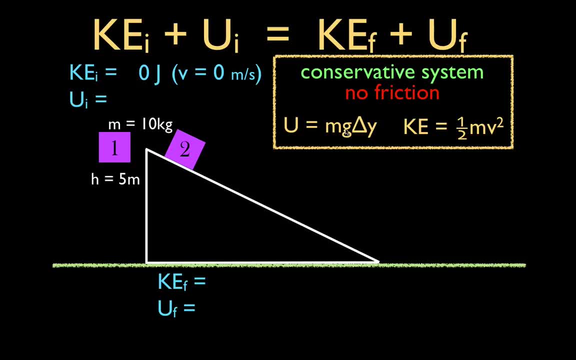 m is the mass, m is 10g. I'm going to round 10 from 9.81 to make the numbers nice and round a little more simple for this example to 10.. And it's 5 meters off the ground. 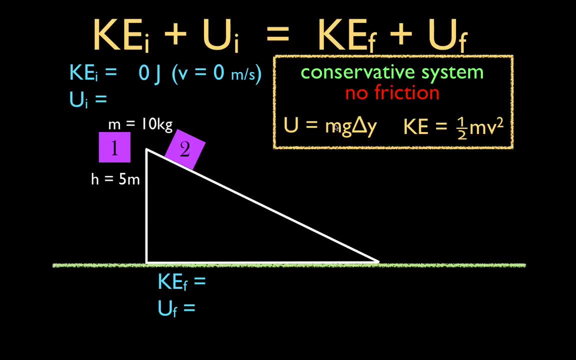 They're both 5 meters off the ground, So each object 10,, 10, and 5,. each object which is 5 meters off the ground has an initial potential energy of 500 joules. Okay, I just want to point out that these objects are standing still no velocity, but they do have some height and therefore they do have no velocity. 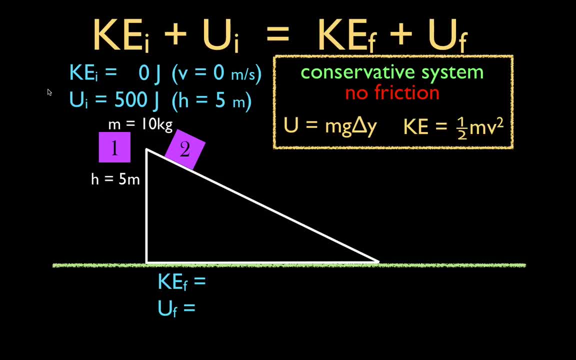 So therefore they're not moving, They have no kinetic energy, but they do have some height and therefore they have some potential energy. Okay, So now I think we're going to let each object fall And as they fall, they're going to pick up velocity, increase their velocity and they're going to fall towards the Earth's surface. 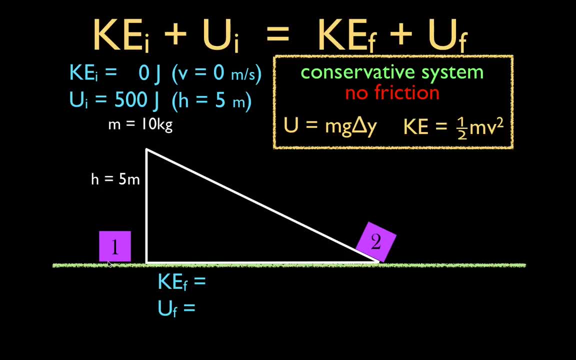 Object 1 falls straight down. no air resistance, And you can see I've stopped it just before it hits the Earth's surface. And therefore this one is going to slide right down and accelerate. no friction, And you can see I've stopped it just before it hits the Earth's surface. 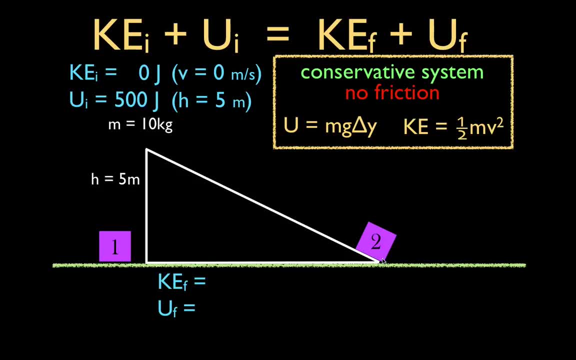 Now we want to see what are the initial- excuse me, the final- kinetic and potential energies of each of these objects. So let's start off with maybe the easier one. I think That's the potential energy, the final potential energy. 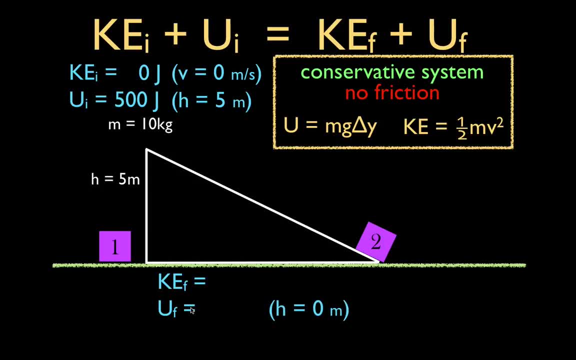 Well, each object now has no height above this surface. So if they have no height, then they have no potential energy. Wow, look, they have no potential energy. Originally they had 500 joules of potential energy in their initial position. 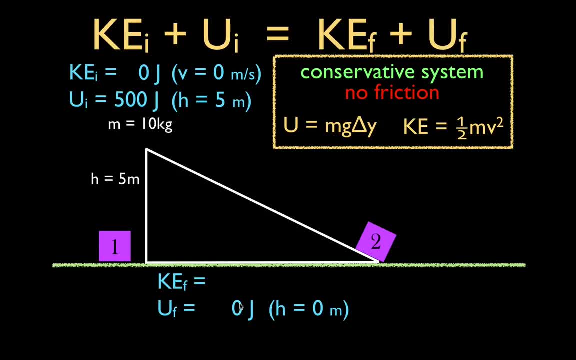 But now they have no potential energy. Well, where did all that 500 joules of potential energy go? Hmm, I wonder. Let's see, we had zero kinetic energy because we had no velocity. But as they fall down, their velocity increases and they gain velocity. 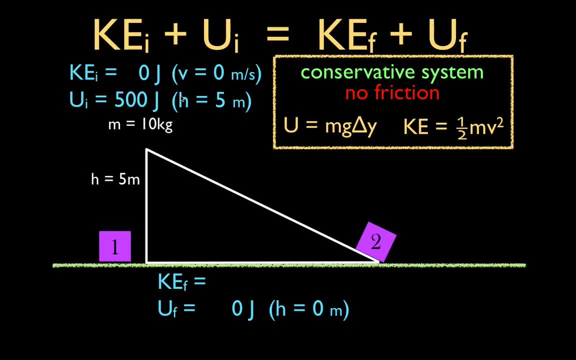 All of their potential energy- because we have conservation of energy- has to be converted into kinetic energy. Okay, Now we know they have a velocity. We don't actually know what the velocity is And sometimes students will say to me: I can't figure out the kinetic energy because I don't know the velocity. 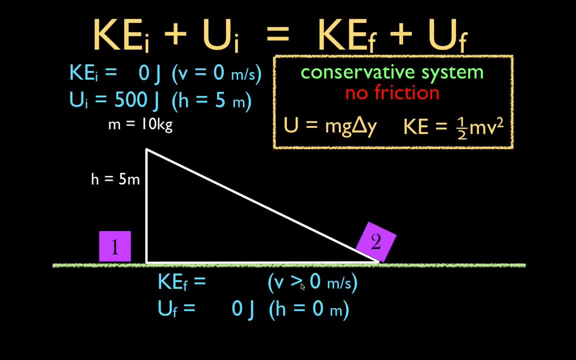 And I say, well, think carefully. If we use conservation of energy, you don't need to know the velocity to figure out the kinetic energy, Because you know you started with 500 joules, Now you have zero for the potential energy. 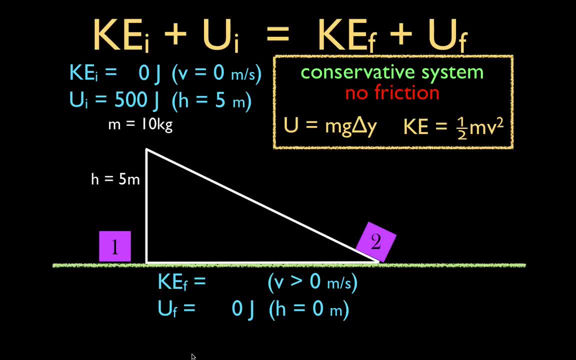 And you started with zero. Well, where did all that go? Where did all that potential energy go? That's right, it went into kinetic energy. Okay, So you can see the initial energy zero plus 500, kinetic plus potential is 500. 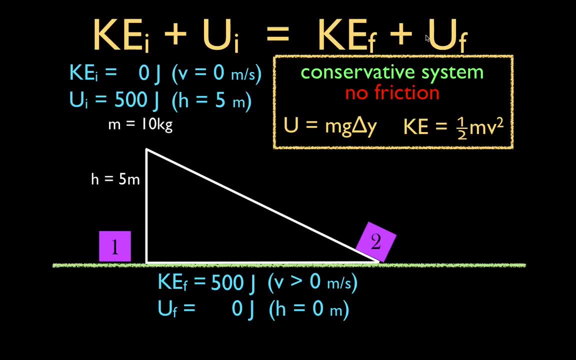 And then the final 500 plus zero, for the final mechanical energy is also 500. So we have conservation of energy Because this is a conservative system, Because we said there's no friction. All right, Now let's think of one other thing really quick here.